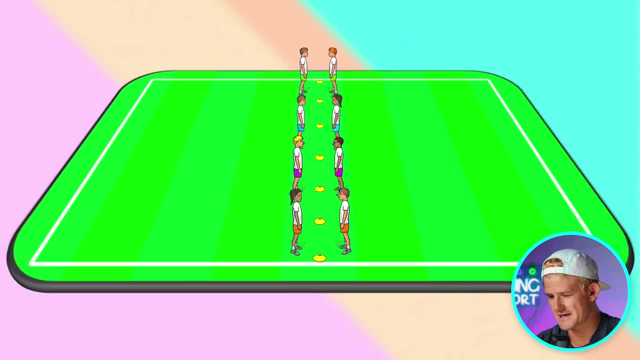 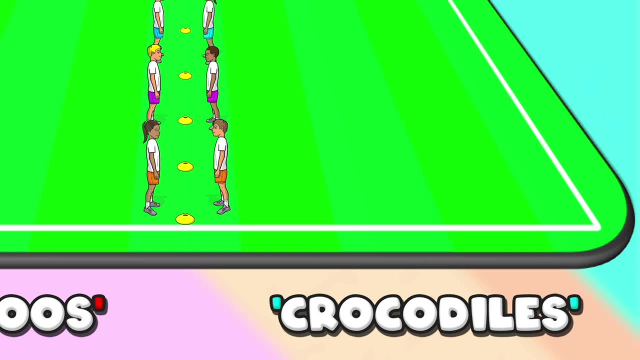 pairs and have them facing each other across that line. Now one side are labeled the kangaroos and the other side are the crocodiles. You can always do any other theme that you like as well. So what's going to happen is everyone's getting ready to run and the teacher calls a side. So 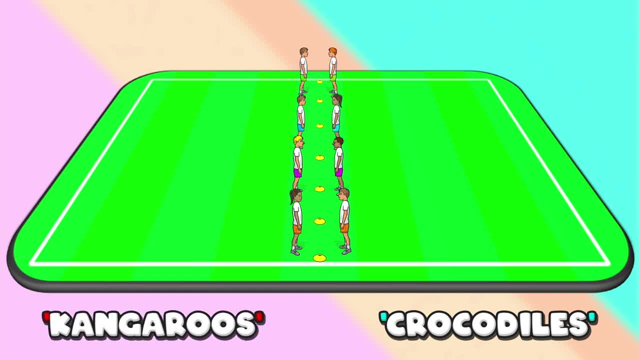 maybe the teacher calls kangaroos. If the teacher calls kangaroos, the kangaroos have to quickly turn and run away to escape from getting tagged by the crocodiles. Now what you can do is you can set up end zones that they have to try and run to, or, for example, they just have 10. 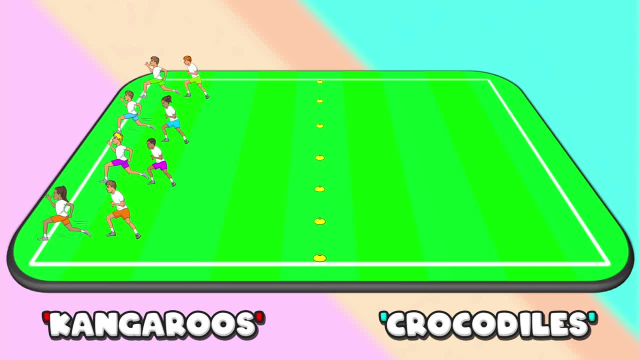 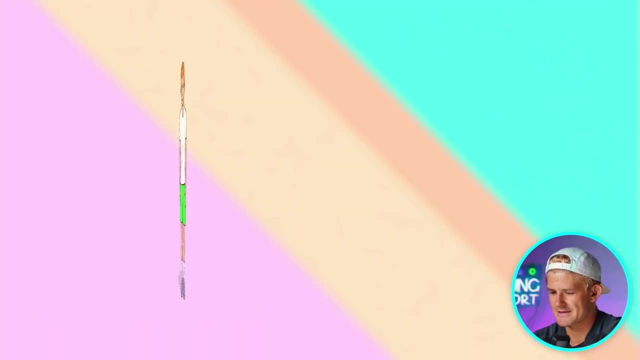 seconds to try and last without getting tagged by their partner. And then you reset. Everyone resets back. This time the teacher calls crocodiles, So crocodiles quickly react and try to run away. So it's very simple, but really good fun. Now what I like to do is I like to call out different 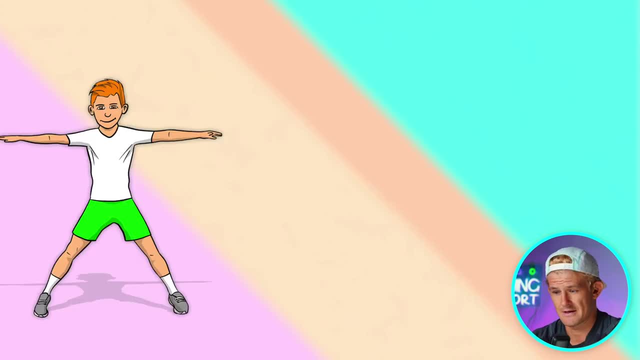 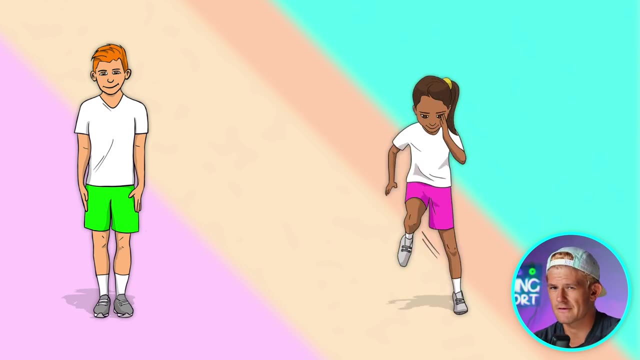 instructions. So maybe before I call out kangaroos or crocodiles, I'll get them to do fitness things like five star jumps, or you can do running on the spot. You can kind of do loads of different things. Whatever you want, Make it creative before they have to quickly run away, and you obviously 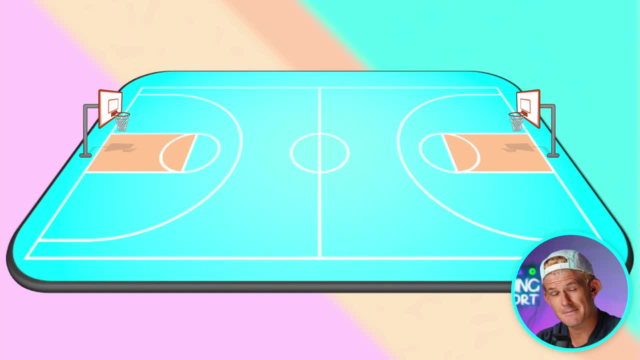 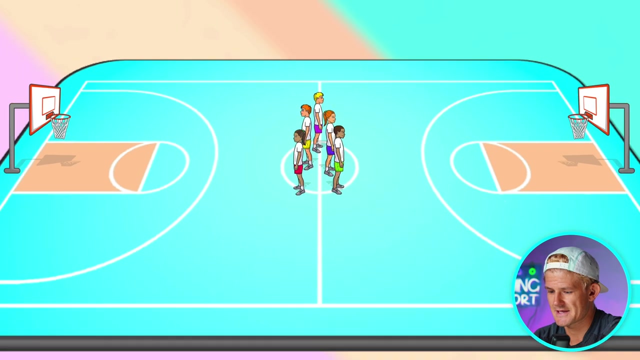 call out a side. The next game is called line elimination, and you can basically play this wherever you have sports court lines or markings. In this example, we're obviously just using a basketball court, So start with everyone in the middle and essentially what's going to happen is: 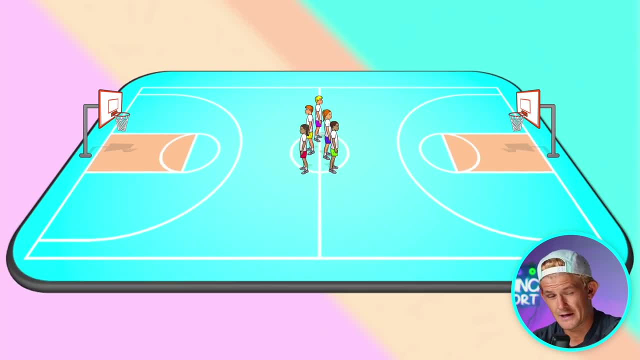 the teacher is going to call out different lines or areas on the court and students have to quickly run there as fast as they can. So in this instance we have side lines that they could call run to. We have base lines. There's the free throw lines. If you're on a volleyball court, maybe you can. 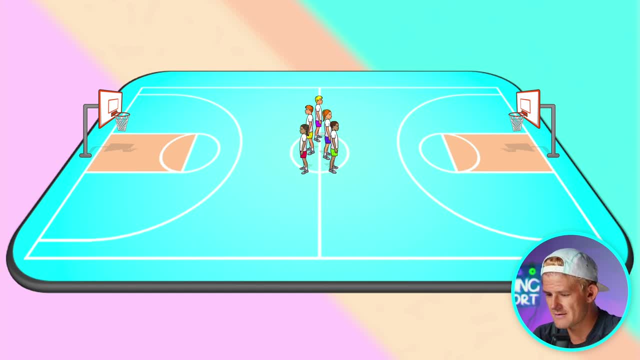 call out the net or even the attack line. So everyone's ready to run, The teacher's got to call out something. So for example, baseline: Everyone quickly runs as fast as they can to stand at any baseline. It can be either end, as long as it's a baseline and the teacher calls out. 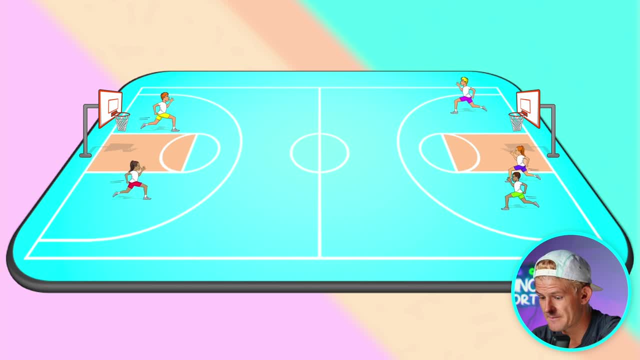 three-point line. So they run to the three-point line and basically, once students are familiar with the lines and the areas of the court, it's good for their learning and understanding. Then you can start to do elimination. So this is where the last player to get to that area or line is out and 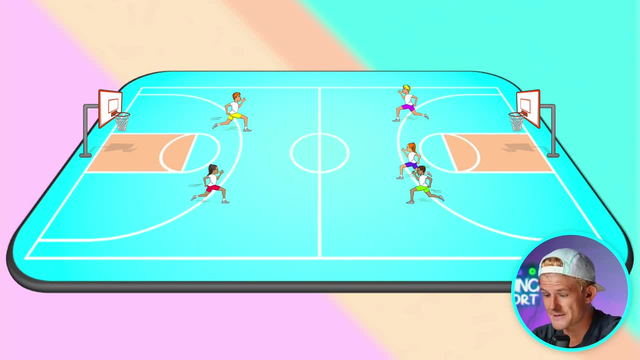 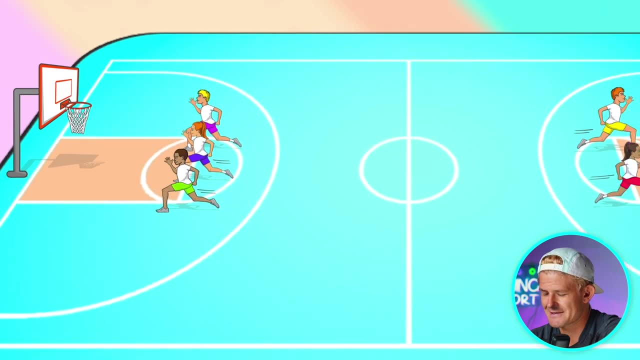 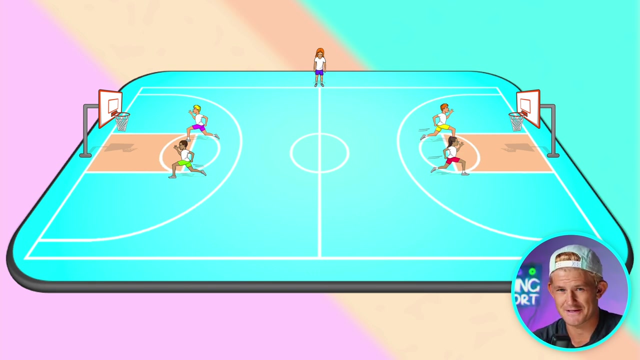 they have to sit on the side. So let's say, the teacher calls out the opposite free throw line. In this instance, you can see that the purple girl was last, So she is eliminated, She goes out to the side and then the gameplay continues and you just keep going until there's a winner. 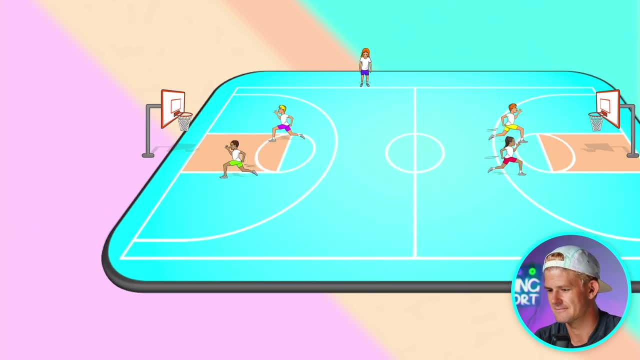 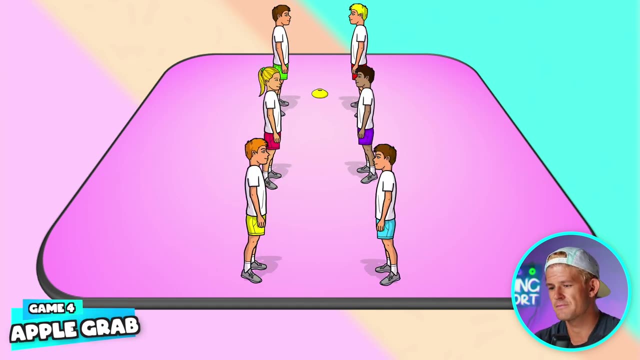 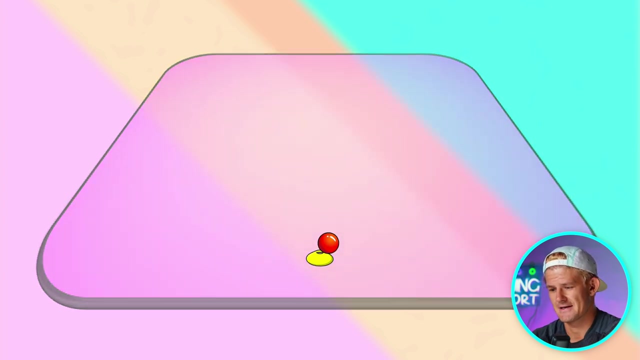 And you can obviously play multiple rounds. The next game is called grab the apple and very simply just get the class into groups of two and each group needs a ball and a cone. So what happens is, when the teacher shouts ball, the first player to quickly grab that ball. who wins, wins a point, and then everyone resets. 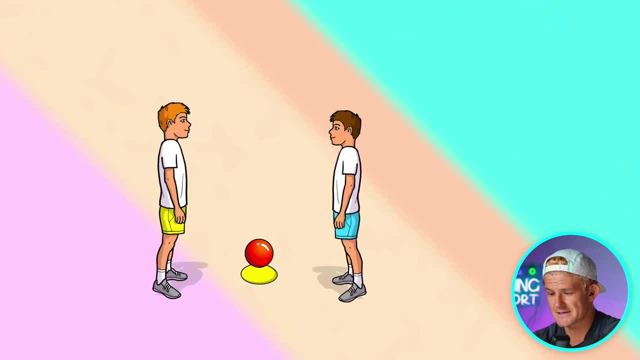 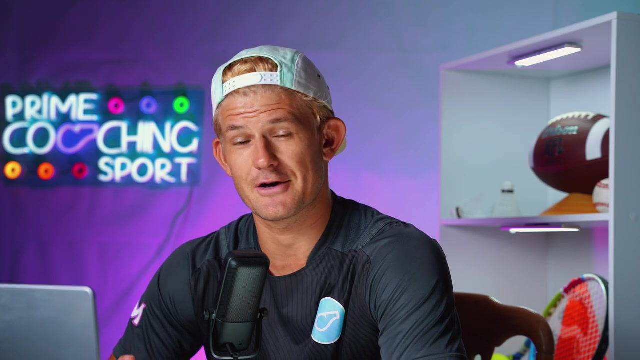 and we go again. Now you can play lots of different variations, so the teacher will call out different instructions. So, for example, they might say: hop on one leg or then get into a crab position before quickly calling ball. So the teachers can be creative as you. 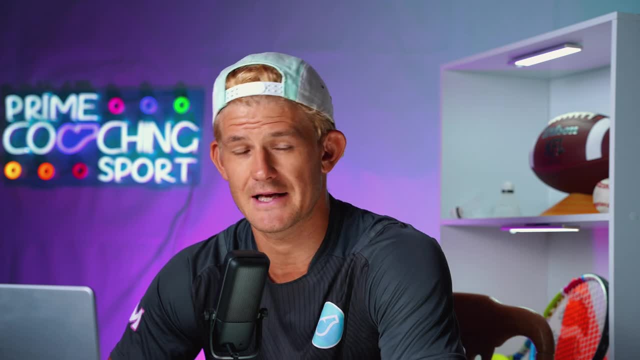 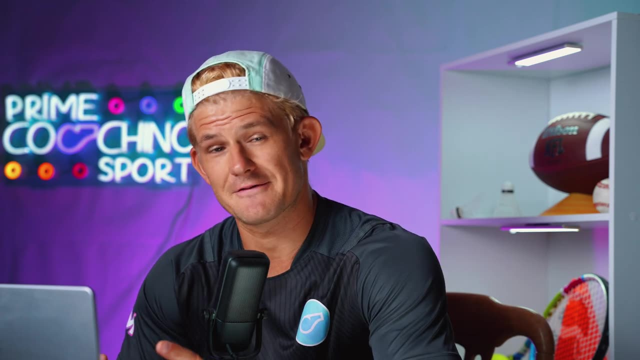 like you can shout out all sorts of crazy things, Get them to spin around, get them to jump around, jump, get them to hop, get them to run on the spot, whatever you can before calling out ball, and they have to quickly react to get that ball. so it's really good fun and you can also vary it. so 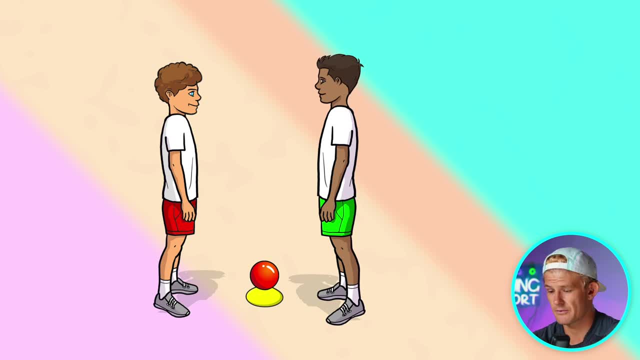 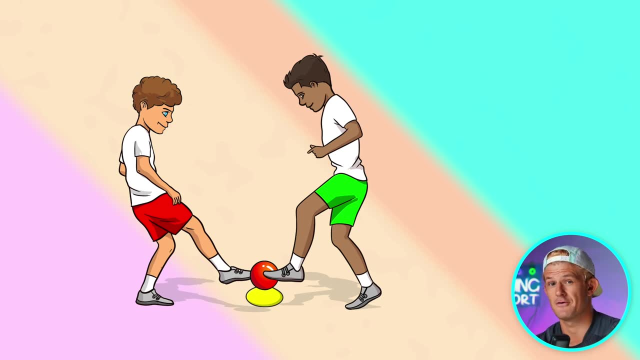 instead of grabbing it with your hands, this time you have to trap it with your foot. so you follow some different instructions and then you have to quickly touch it with your foot. the first one to put their foot on top of the ball wins. you can get points going. you can have the pair switch. 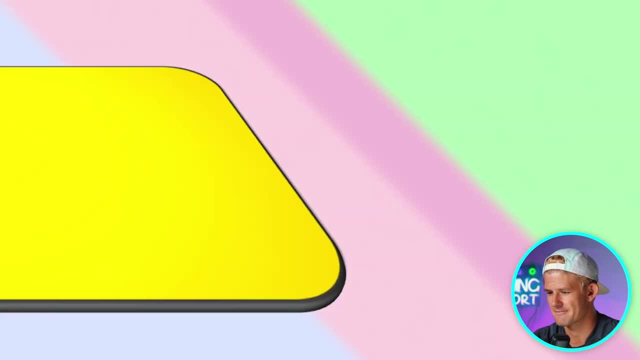 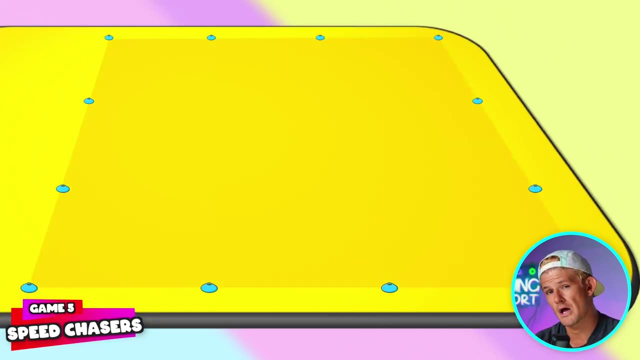 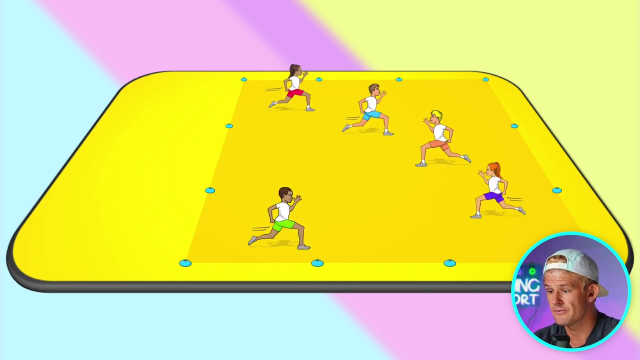 all sorts of things like that. the last game is called speed chases and for this, just using cones, you're going to mark out a large area and that area is going to be the tag zone. now, inside the tag zone, you're going to put five or ten dodgers, depending on the class size. larger classes you'll. 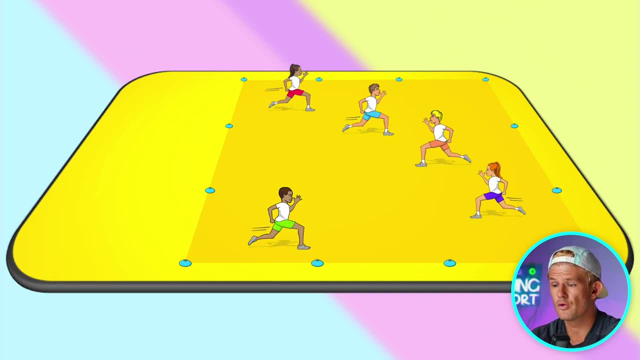 have more smaller classes. you might have less. you'll get an idea of how many you need in there once the game gets going. you and then the rest of the class are going to line up on the side. they are the chasers or the taggers. so we've got two groups, we've got the taggers and we've got the dodgers. 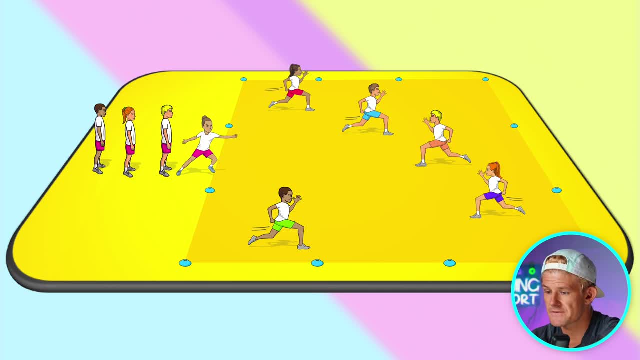 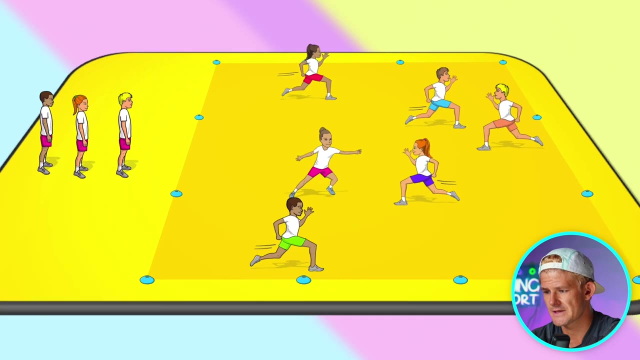 so when the teacher blows the whistle, the chaser at the start of that line has 10 seconds to tag as many people as they can. everyone has to stay within that square. you can't leave it and they're trying to tag as many as they can to be eliminated. so let's say: this girl tags the other girl that. 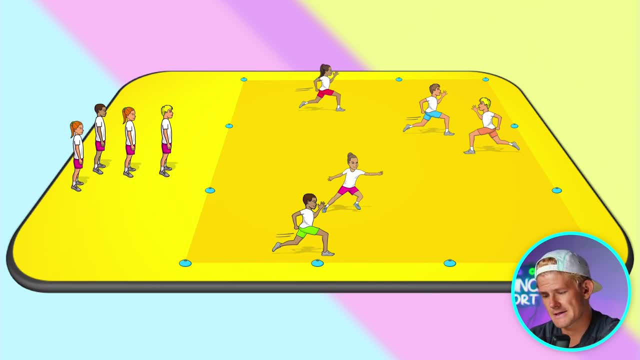 girl who was the first to tag the other girl, and she's going to tag the other girl and she's going to tag them. she's going to take over. so she's going to be the chaser. she'll go in and hold the chaser and then she'll come in. that way just be like one person. the rest of the Auckland. 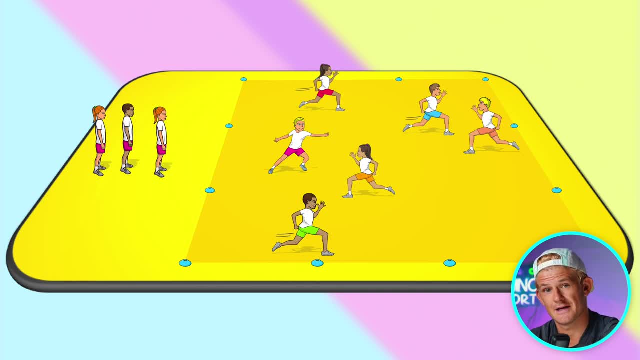 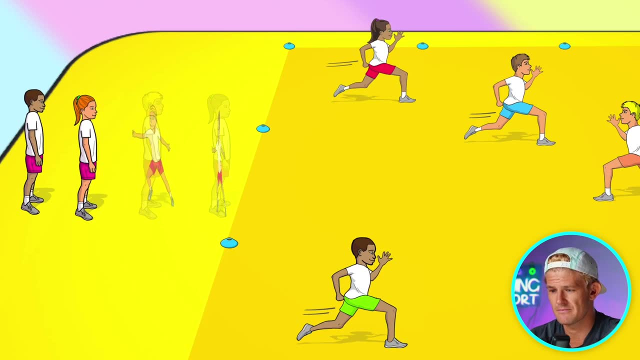 it could be five people. they have to come out of that square and join the chasing line. you can then adapt it so instead of just one chaser at a time line, so when you're in the way of the chasing line, on top of that you have to take all five chasers. 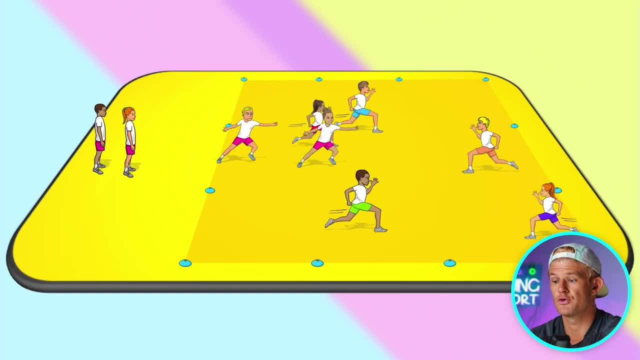 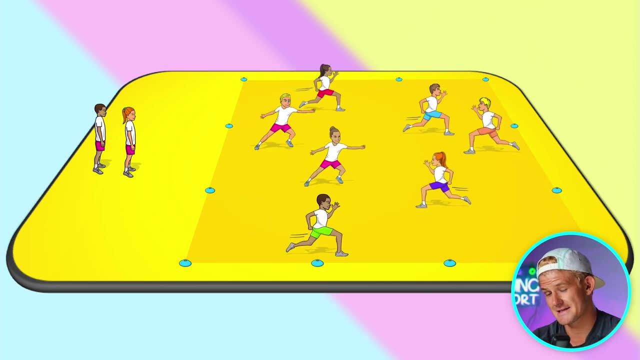 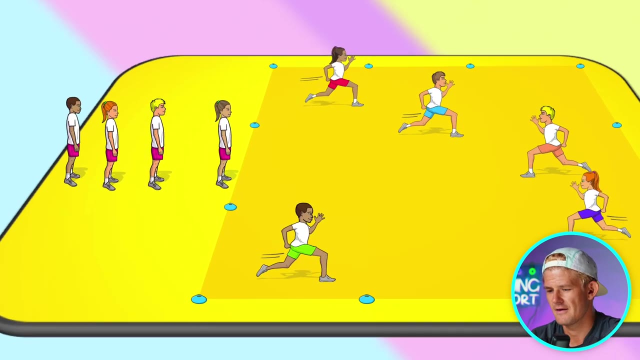 have two people coming in, so it might be even harder this time. two people coming in trying to eliminate and tag as many as possible before the time is up and teacher blows the whistle. so it's a continuous ongoing tagging game all the time. you can even vary it, where this time the tagger has a noodle. i think this is really good fun and 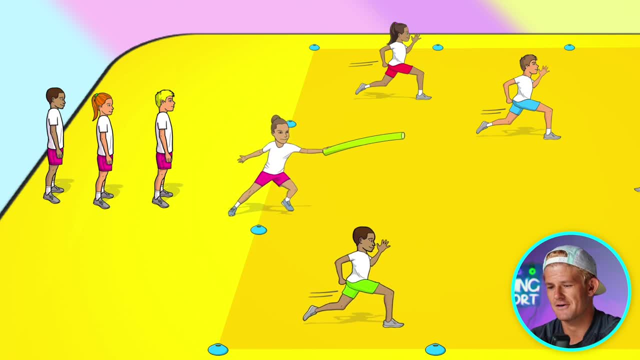 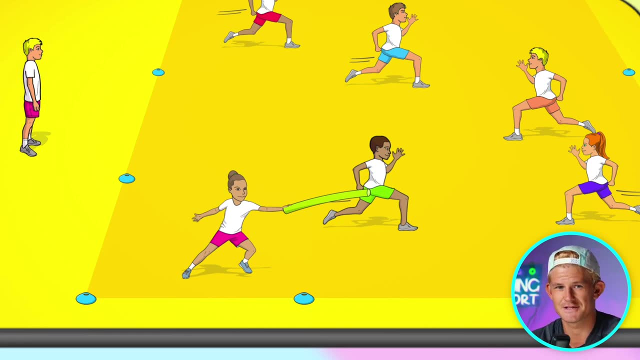 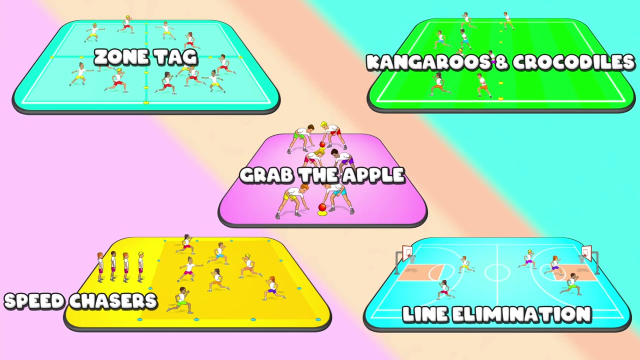 it's safe as well. using the long foam noodle they have to try and tag people, making sure it's below the waist. so it's safe as well. it's a good variation to the typical tagging escaping kind of game. so there you have it. those are all the instant pe games for now. i've got so many more. 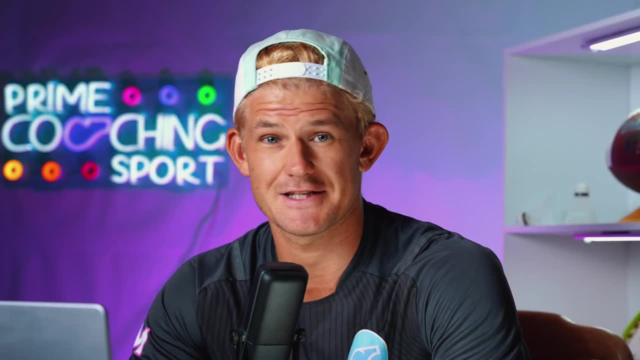 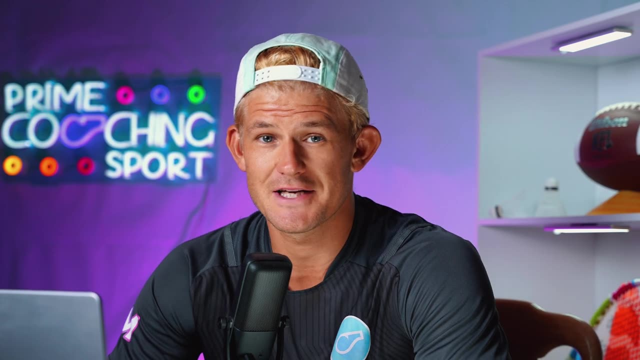 ideas that you can choose from. i've got complete lesson plans, complete sports units. this was just a brief introduction to some of the games that i have. make sure you check out my lesson plans in the links below and i'll see you in the next one. bye. see you next time for some more game changing sport.